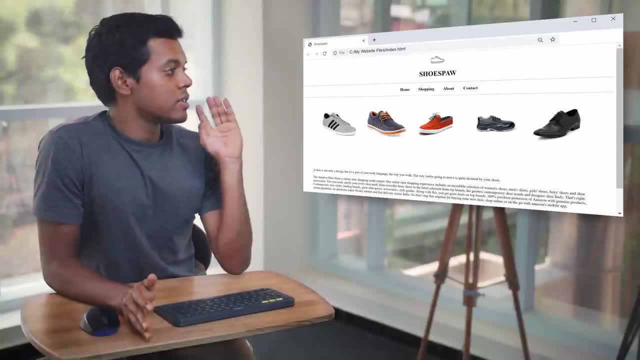 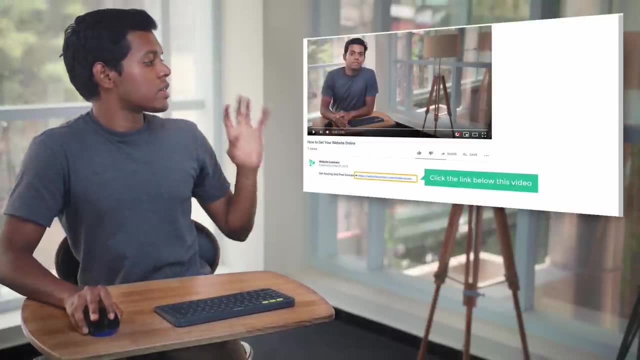 So once you have your files ready, we can now get started. So we are going to get this website online in just four steps. The first step is to choose your website name. Okay, So to choose your website name, just click the link below this video and it'll take you. 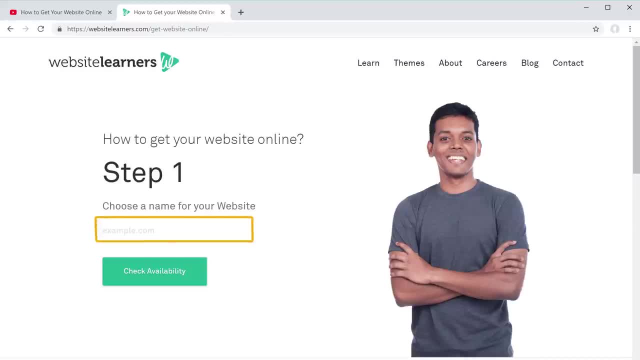 to this page Now choose any name you want and then enter it here. So I'm going to enter my website name as shoespotcom and then click check availability. So, as you can see, this name is available. So once you get the name, 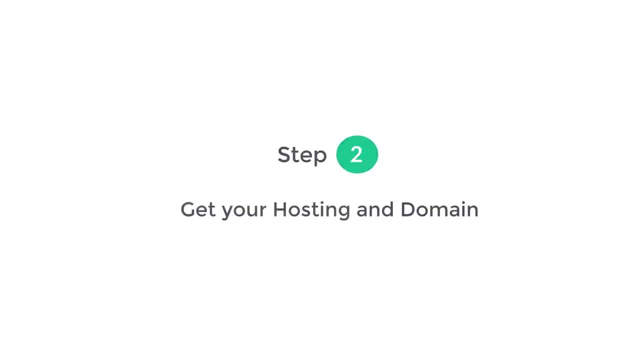 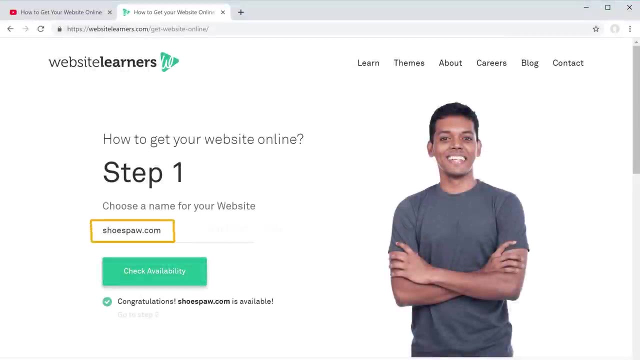 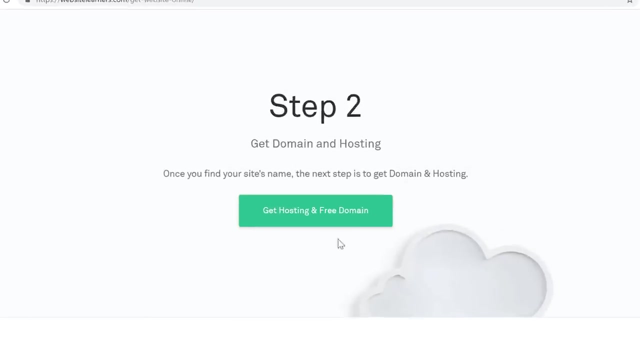 You can go to the next step, which is to get your hosting and domain. So hosting is a place where your website's files will be stored and domain is your website's name. So to get this domain name and hosting, just scroll down this page and click get hosting. 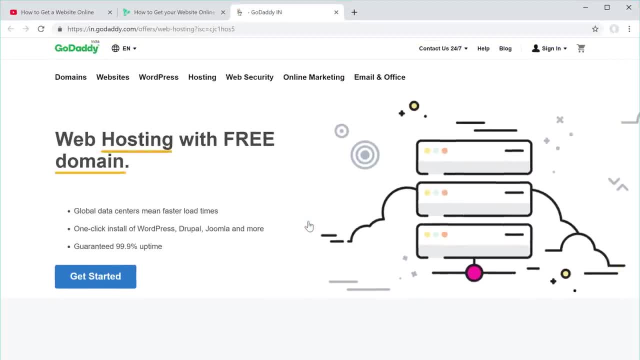 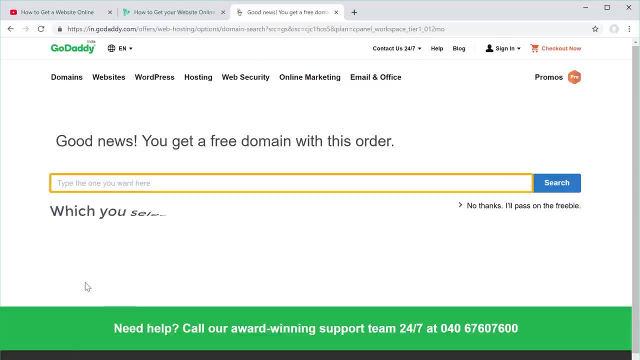 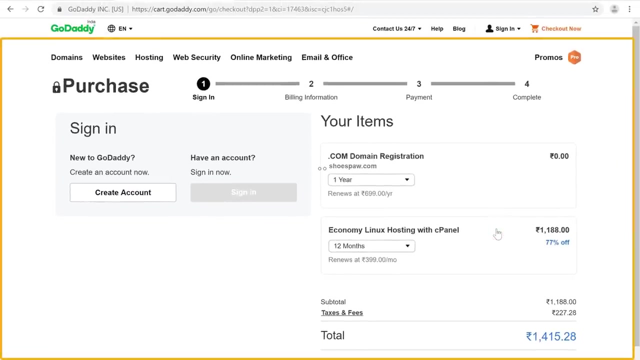 Now this will take you to godaddycom where we are going to get the hosting and domain. So to get it, let's click get started. Okay, Now enter the same name which you selected before and click search, then click select and continue, and now it'll take you to this card page. 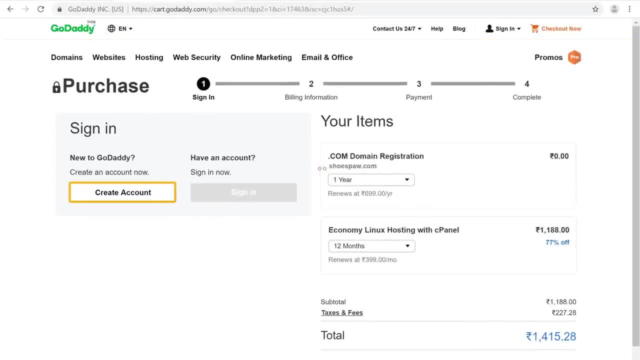 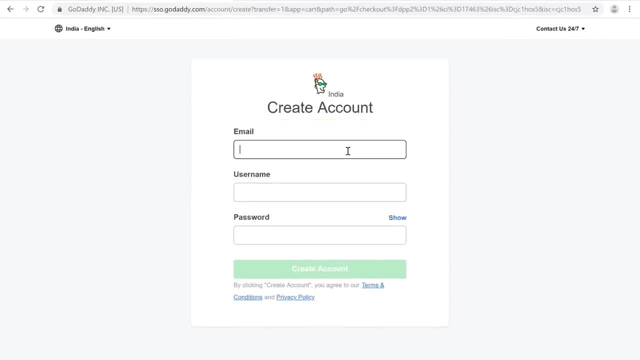 Now, to get the domain and hosting, we need to create a new account. So let's click here and then fill up these details and click create a new account. Okay, So let's go ahead and create a new account. So let's go ahead and create a new account. 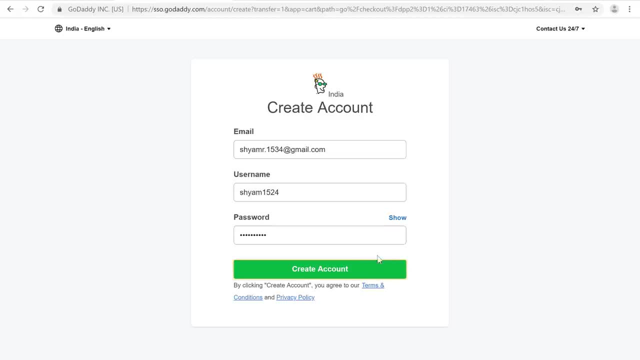 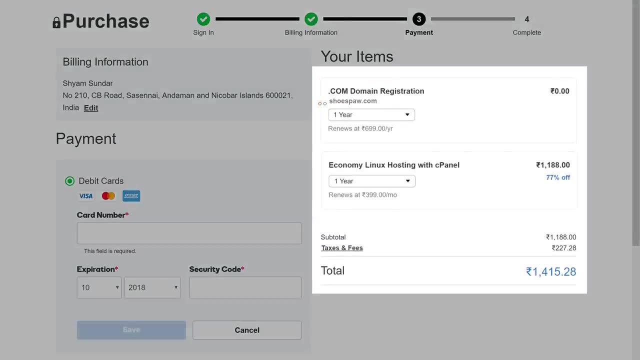 So let's click here and then fill up these details and click create a new account. Okay, So let's go ahead and create a new account. So let's go ahead and create a new account Now. here you can see that we are getting our domain, which is shoespotcom, and our hosting. 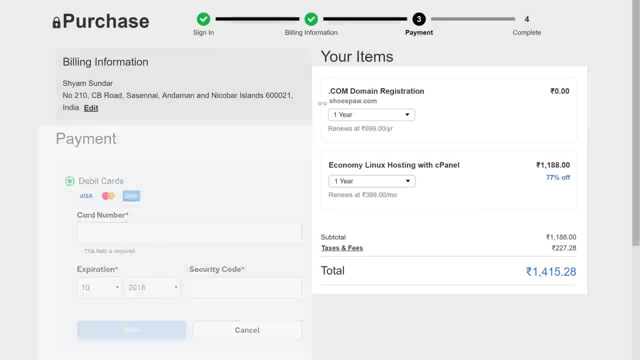 Now, both of these are going to be valid for one year, So this means once we place this order, your website will be live on the internet for the next one year. Now let's go ahead and make the payment. Just choose your payment method, enter your details and then click save and then complete. 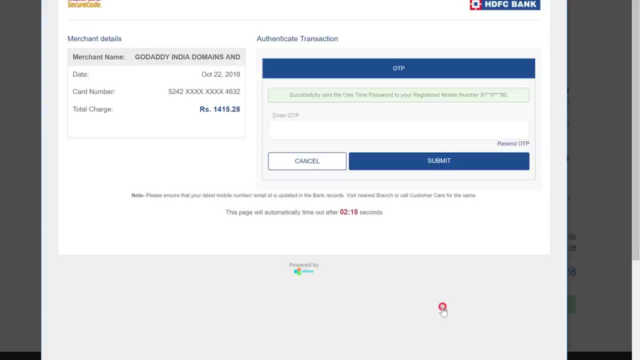 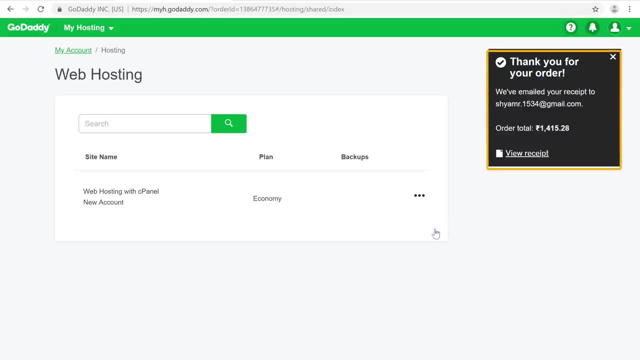 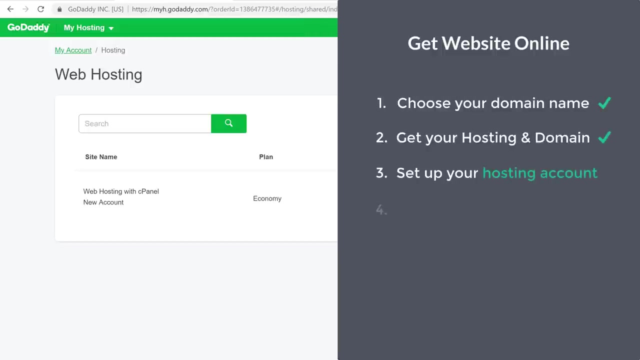 this purchase. okay, so now we have successfully made our payment and we have got our domain and hosting. so once you've got your hosting and domain, you can go to the next step, which is to set up your hosting account. so once you set up your hosting account, you'll be able to upload your website. 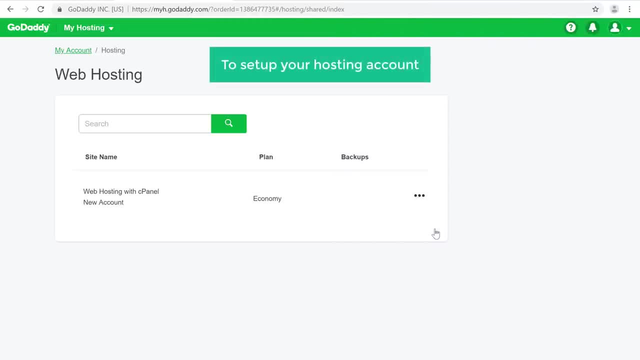 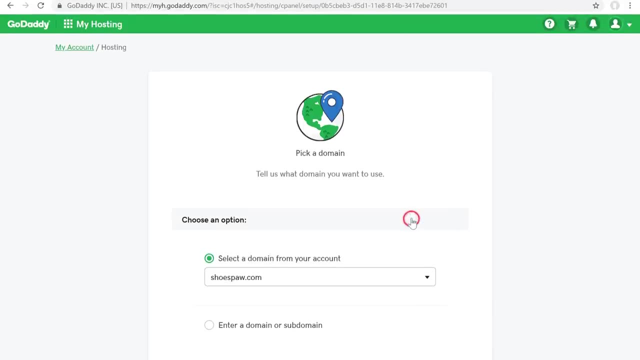 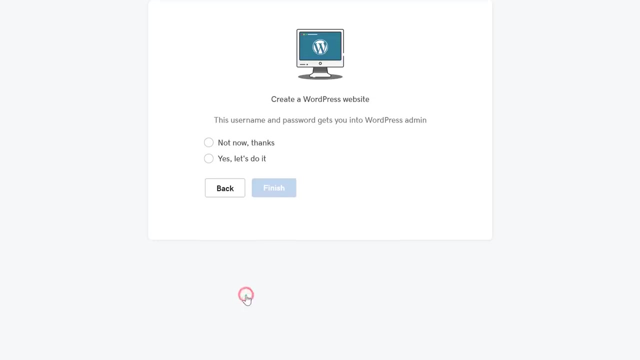 files. so to set up your hosting account, just click here and click set up now, click Next and then again next. now skip this step by clicking not now and then click finish. so now we have set up our hosting account. so let's click go to dashboard. so once you set up your hosting account, you can go to the next step, which is to set up your hosting account. so once you set up your 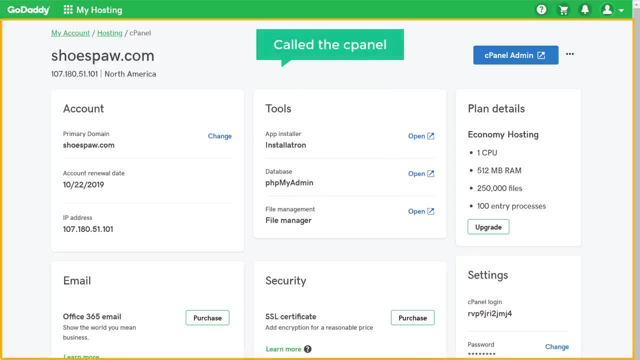 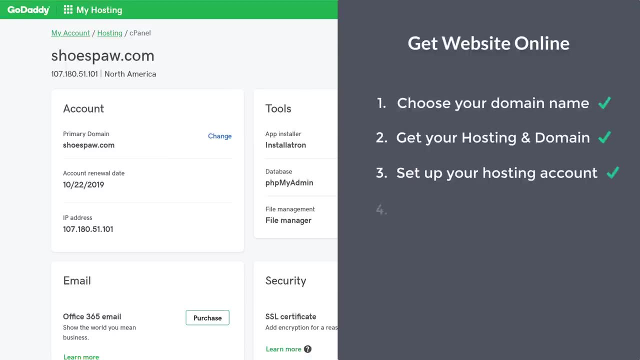 hosting account, you will reach this page called the cPanel, so this is the place where you can control your hosting account. so once you reach this page, you can now go to step 4, which is to upload your website files to this hosting account. so once you upload the website files, your website will be live on the 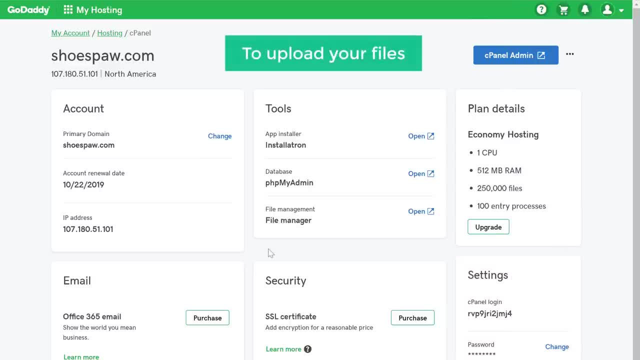 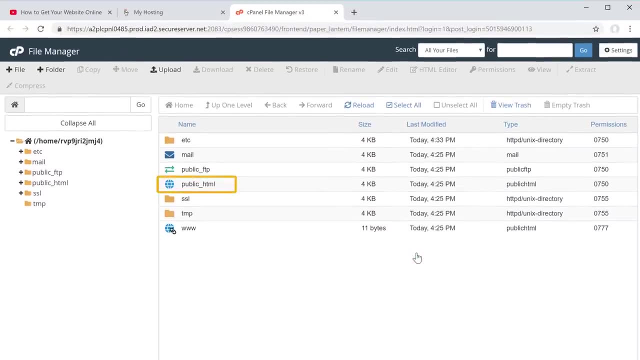 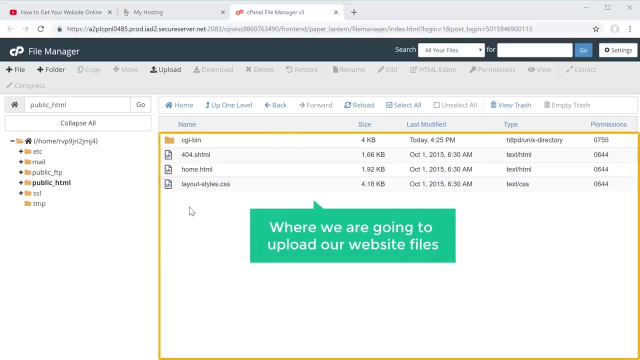 internet. so to upload your files, just click open next to File Manager. you so 1 click. the public is Joseph. Now this is the place where we are going to upload our website files Now we have a few sample files here. Now, before we upload our files, let's delete these sample files. 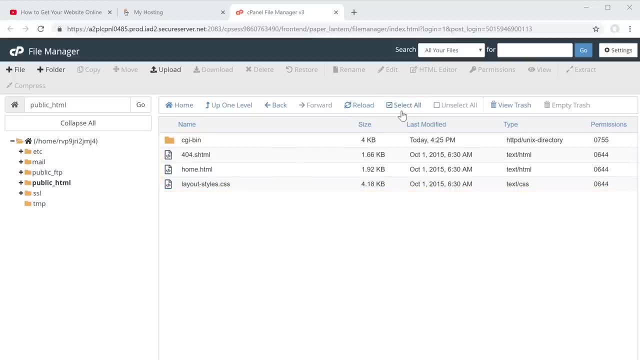 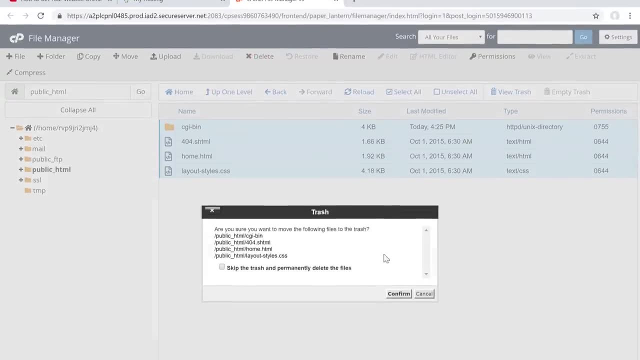 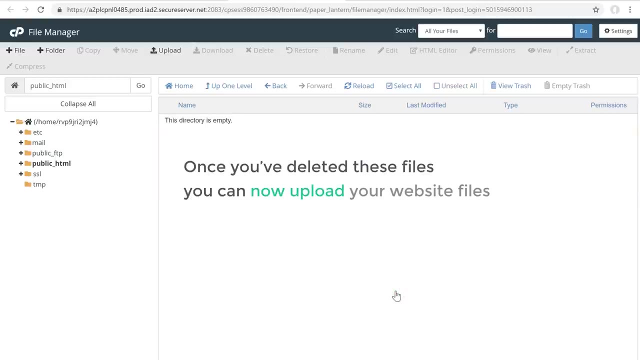 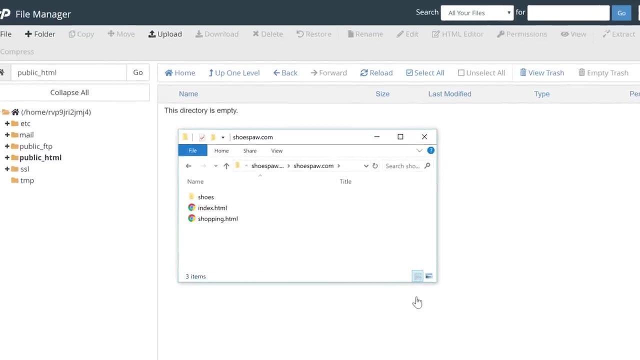 So to delete it, let's first click select all and then click delete, Now click confirm and all the files will be deleted. So once you've deleted these files, you can now upload your website files. So to upload our files, let's open the folder which has our HTML files. 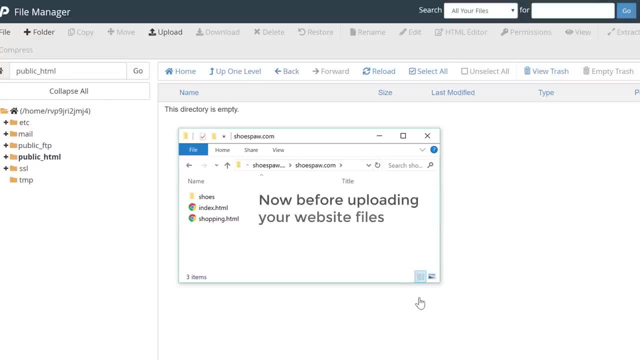 So these are the website files which I'm going to upload Now. before uploading your website files, make sure your homepage is named as indexhtml. So, once you have these files ready, instead of uploading them one by one, we are going to compress them into one file. 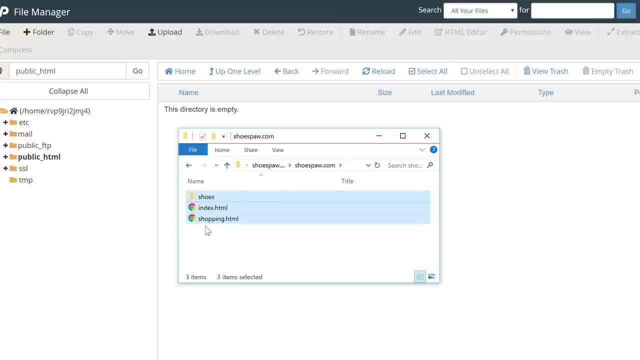 So to compress it, let's select all the files And then right click and go to send to and click compressed file, And now you'll get this zip file which will have all your website files. Now to upload this zip file, let's go back to our hosting page and then click upload. 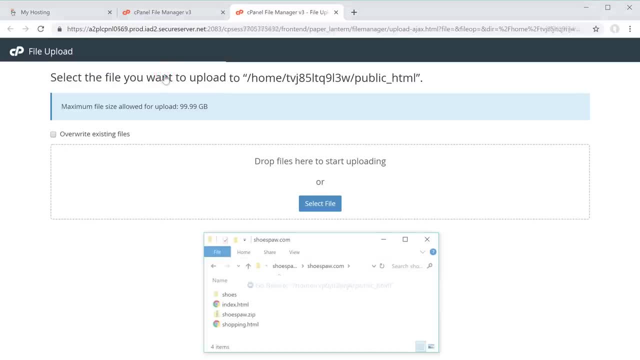 here Now. just drag the zip file from your computer and then drop it here, And the first thing that you need to do is to go to your website. So let's go to our website. Let's go to our website And then click download.